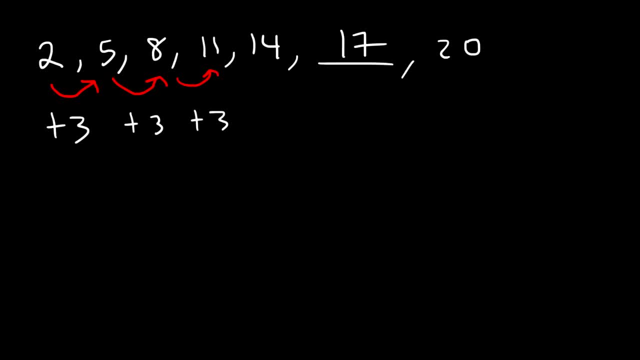 17 plus 3 will give us the next number, 20.. So anytime you have a sequence that differs by repeated addition or subtraction, it's an arithmetic sequence. Now let's work on another example. Let's say if we have these numbers- 5,, 9,, 13,, 17.. 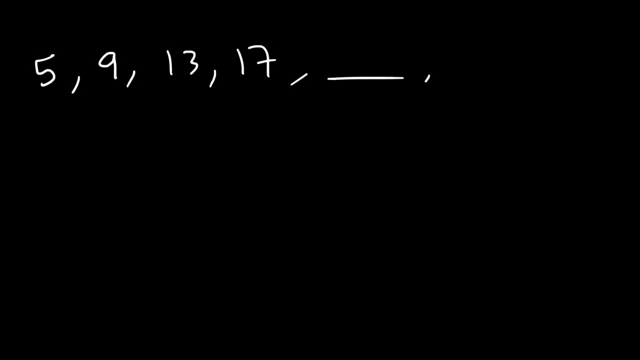 What's the next number in the sequence? Find the next three numbers actually. Feel free to pause the video. So notice that 5 differs from 9 by 4 units. If we add 4 to 5, it will give us 9,, and if we 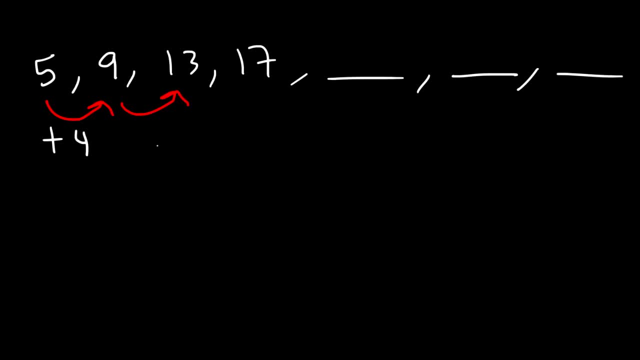 add 4 to 9, it will give us 13.. So therefore the common difference is 4.. So to find the next number in the sequence, we need to add 4 to 17.. 17 plus 4 is 21.. 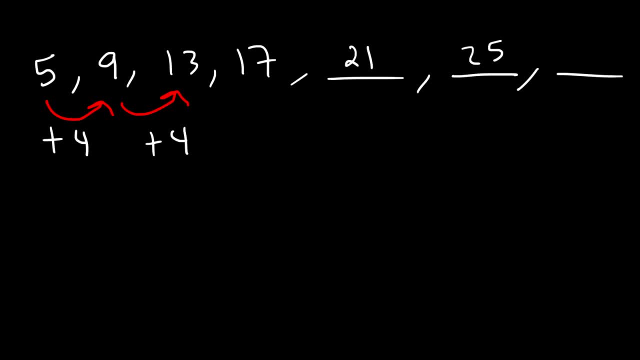 Twenty-one plus four is twenty-five, and then twenty-five plus four is twenty-nine. Here's a different example: Twenty-seven, twenty-one, fifteen and then nine. Find the next three terms in the sequence. So what is the common difference? 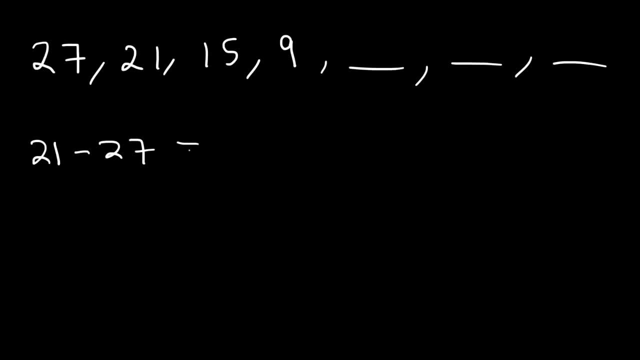 If we take the second number and subtract it by the first number, we're going to get negative six. If we take the third number and subtract it by the second number, it will give us the same number: negative six. So therefore, the common difference is negative six. 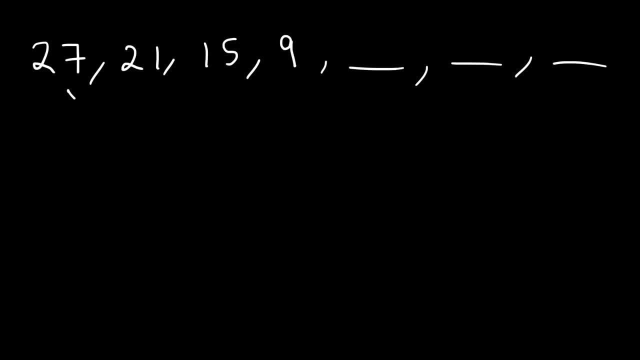 So if you add negative six to twenty-seven, you're going to get twenty-one. And if you add another negative six to twenty-one, it will give you fifteen. Or if you subtract twenty-one by six, you get fifteen. Fifteen minus six is nine. 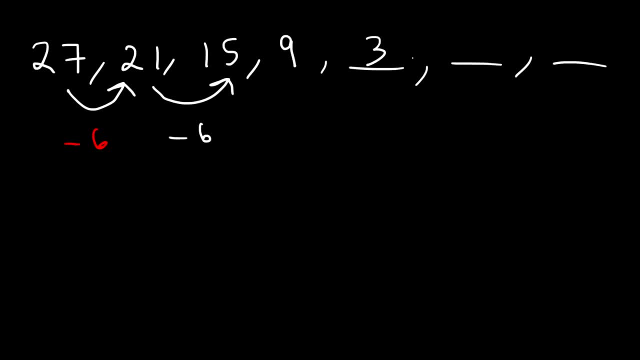 Nine minus six will give us the next number three, And then three minus six will give us negative three, And then negative three minus six will give us the last number, negative nine. So the common difference is negative six. Once you have that, then you can find the next term in the sequence. 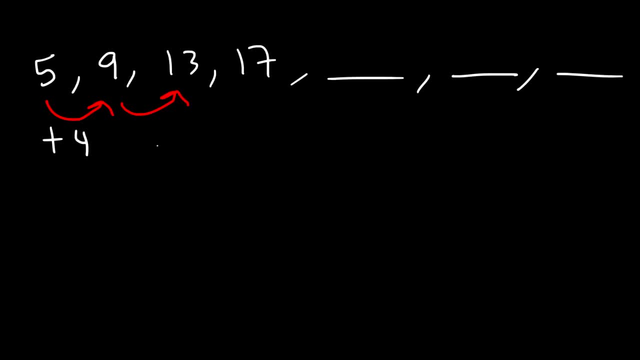 add 4 to 9, it will give us 13.. So therefore the common difference is 4.. So to find the next number in the sequence, we need to add 4 to 17.. 17 plus 4 is 21.. 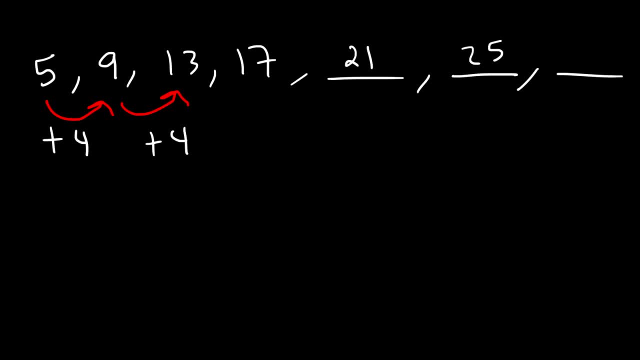 21 plus 4 is 25 and 25 plus 4 is 29.. Here's a different example: 27,, 21,, 15 and then 9.. Find the next three terms in the sequence. So what is the common difference? 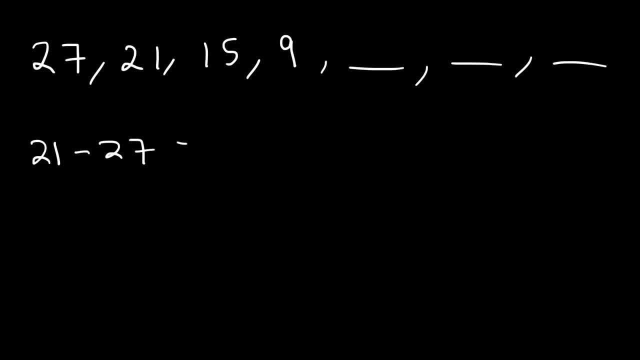 If we take the second number and subtract it by the first number, we're going to get negative 6.. If we take the third number and subtract it by the the second number, it will give us the same number, negative 6. so therefore the common difference is negative 6. so if you add negative 6 to 27, you're gonna 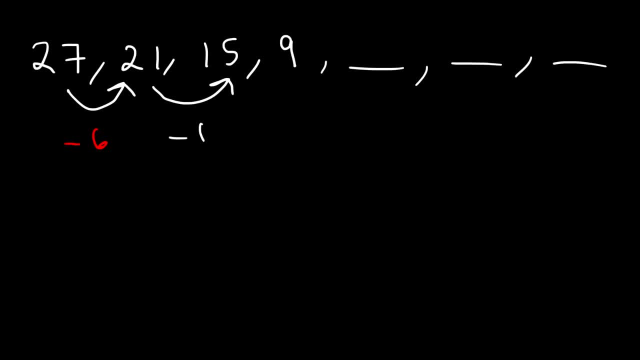 get 21, and if you add another negative 6 to 21, it will give you 15, or if you subtract 21 by 6, you get 15. 15 minus 6 is 9. 9 minus 6 will give us the next. 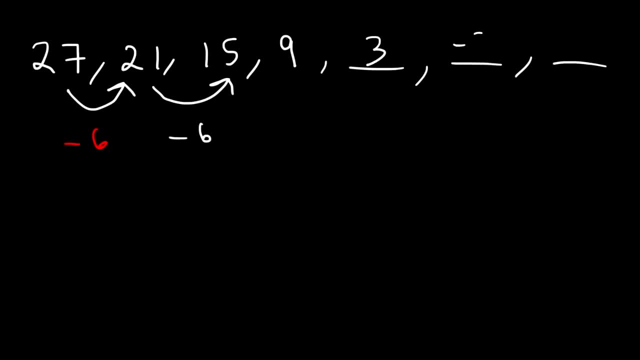 number 3, and then 3 minus 6 will give us negative 3, and then negative 3 minus 6 will give us the last number, negative 9. so the common difference is negative, since once you have that and then you could find the next term in the sequence. 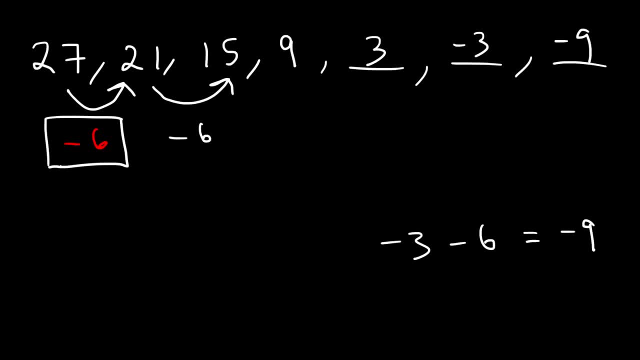 so once again, this is another arithmetic sequence or arithmetic sequence. here's the next sequence. here's a different problem. to try, let's say, if we have the sequence 3, 6, 12 and 24, what is the next number in the sequence? so first let's see if there's a. 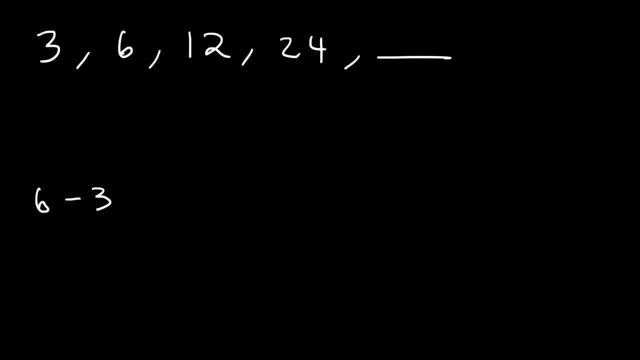 common difference. if we take the second term and subtract it by the first term, it will give us a difference of three, and if we take the third term and subtract it by the second, we're gonna get a difference of six, and so that's not gonna help as much. 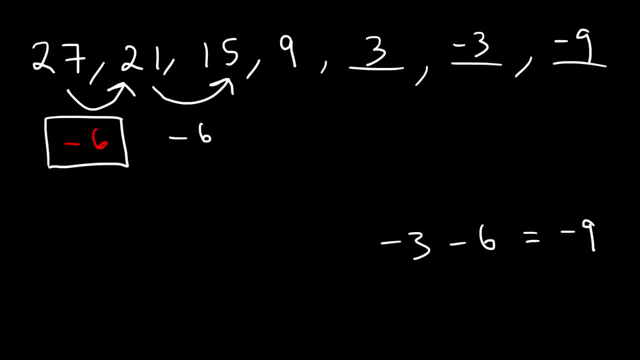 So once again, this is another arithmetic sequence. Here's a different problem. to try, Let's say, if we, Let's say we have the sequence three, six, twelve and twenty-four, What is the next number in the sequence? So first let's see if there's a common difference. 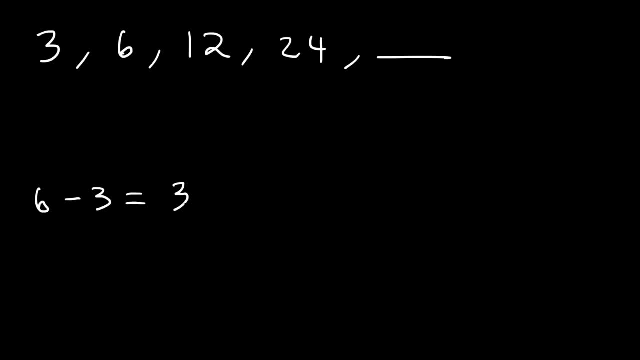 If we take the second term and subtract it by the first term, it will give us a difference of three, And if we take the third term and subtract it by the second, we're going to get a difference of six, And so that's not going to help us much. 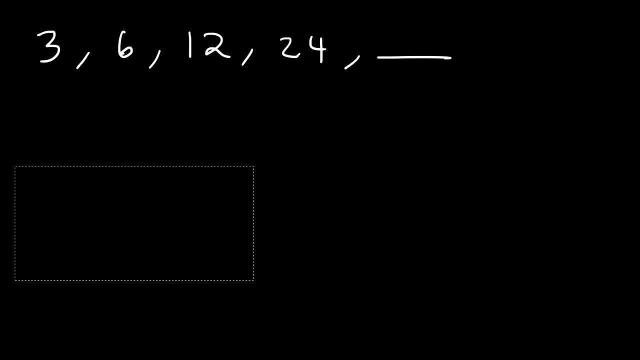 But let's divide the second term by the first term. Six divided by three is two, And if we take the third term divided by the second, we will get two. So therefore, this sequence has a common ratio of two. Notice that to get from three to six, or to go from three to six, we'll need to multiply by two. 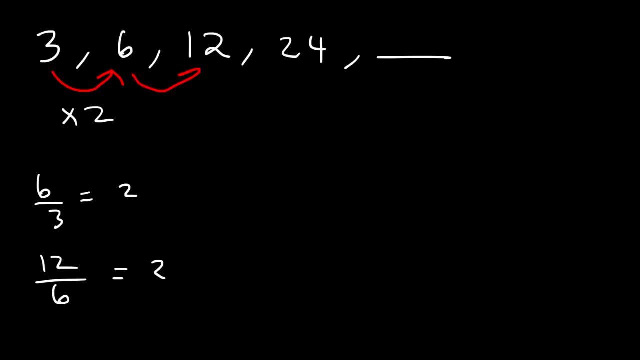 Three times two is six. And if we multiply six by two, that will give us twelve. And then if we multiply twelve by, If we multiply twelve by two, it will give us twenty-four. So this is what's known as a geometric sequence. 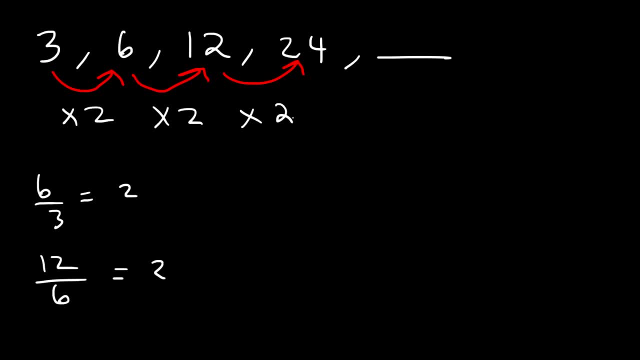 Because the numbers they differ by multiplication or division, as opposed to addition and subtraction. So to find the next number in the sequence, we've got to multiply twenty-four by two, which will give us forty-eight. And then, if we want to find the next one, it's going to be forty-eight times two, which is ninety-six, and so forth. 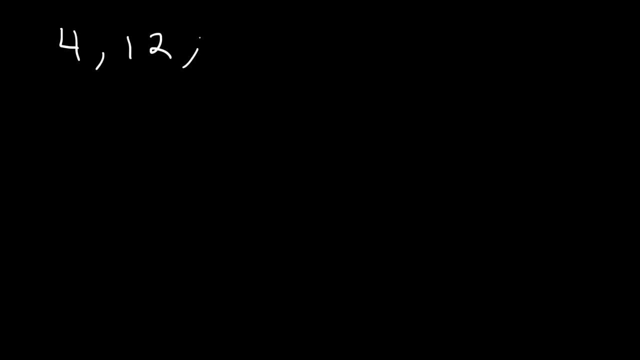 Here's another. Let's take a similar example. Let's say, if we have the numbers four, twelve, thirty-six, What is the next number in the sequence? So let's see if it's an arithmetic sequence or a geometric sequence. Let's see if there's a common difference. 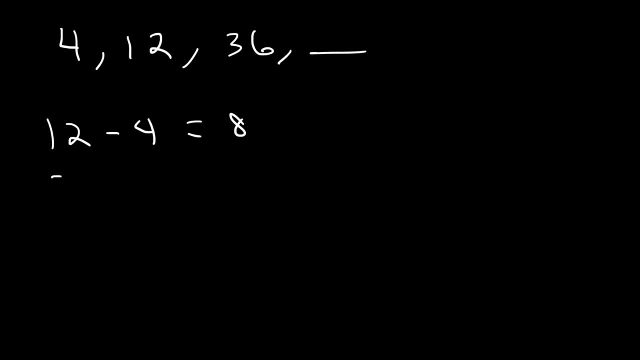 If we take the second term and subtract it by the first, we'll get eight, And if we take the third and subtract it by the second, this will give us twenty-four. So therefore we don't have an arithmetic sequence. Let's test to see if it's a geometric sequence. 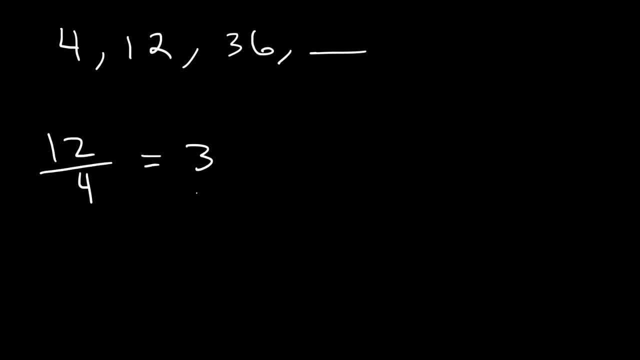 Twelve divided by four will give us three, and thirty-six divided by twelve is three. So we have a common ratio. If we multiply four by three, it will give us twelve, And if we multiply twelve by three, that will give us thirty-six. 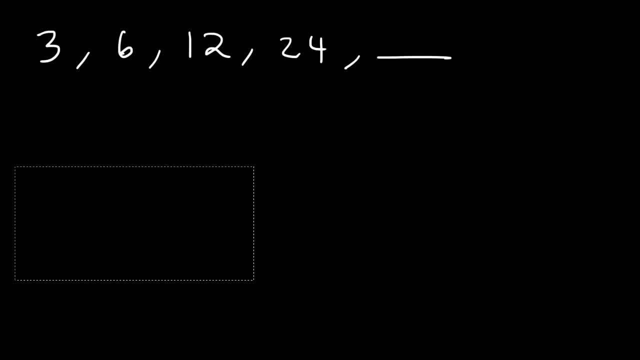 but let's divide the second term by the first and then the second term by the first. n- this is not a term by the first term. 6 divided by 3 is 2, and if we take the third term divided by the second, we will get 2.. So therefore, this sequence has a common ratio of 2.. 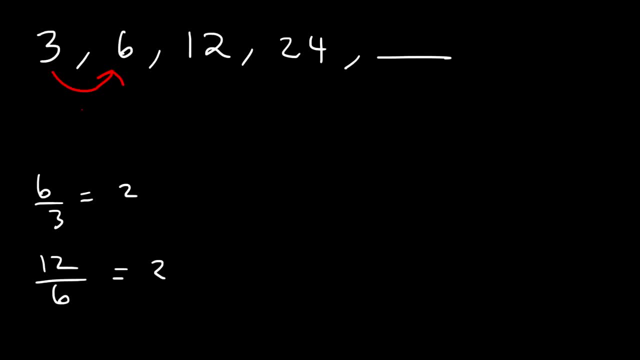 Notice that to get from 3 to 6, or to go from 3 to 6, we'll need to multiply by 2.. 3 times 2 is 6, and if we multiply 6 by 2, that will give us 12,, and then, if we multiply, 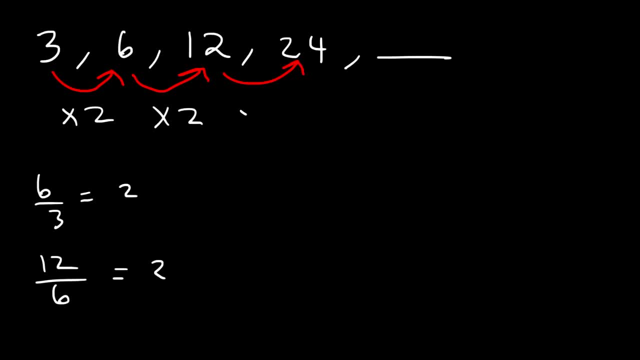 12 by 2, it will give us 24.. So this is what's known as a geometric sequence, because the numbers they differ by multiplication or division, as opposed to addition and subtraction. So to find the next number in the sequence, we've got to multiply 24 by 2, which will 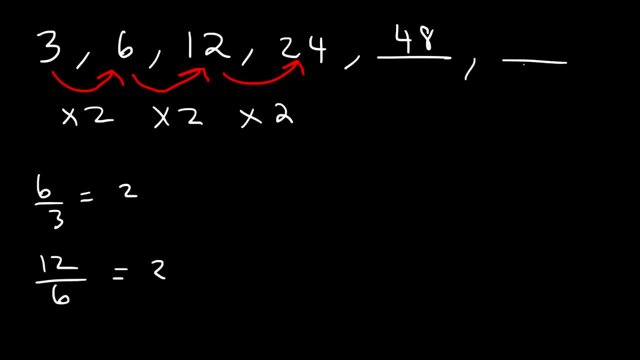 give us 48. And then, if we want to find the next number in the sequence, we've got to multiply 24 by 2, which will give us 48. And if we want to find the next one, it's going to be 48 times 2, which is 96, and so 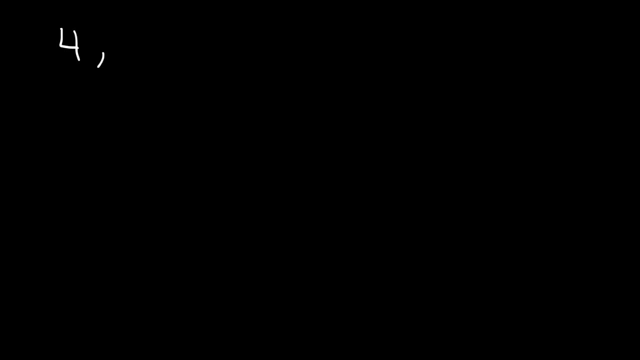 forth. Here's another similar example. Let's say, if we have the numbers 4,, 12,, 36, what is the next number in the sequence? So let's see if it's an arithmetic sequence or a geometric sequence. Let's see if there's a common difference If we take the second term and 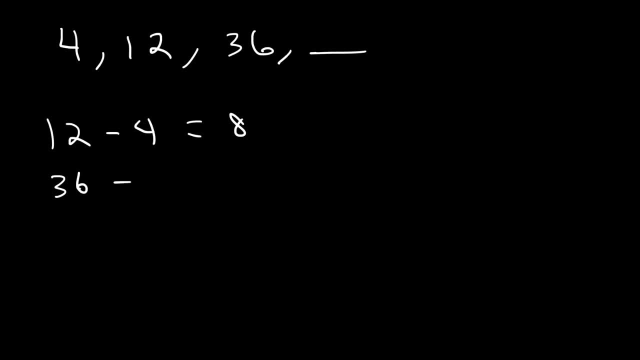 subtract it by the first, we'll get 8.. And if we take the third and subtract it by the second, this will give us 24.. So therefore, we don't have an arithmetic sequence. Let's test to see if it's a geometric sequence: 12 divided by 4 will give us 3, and 36 divided. 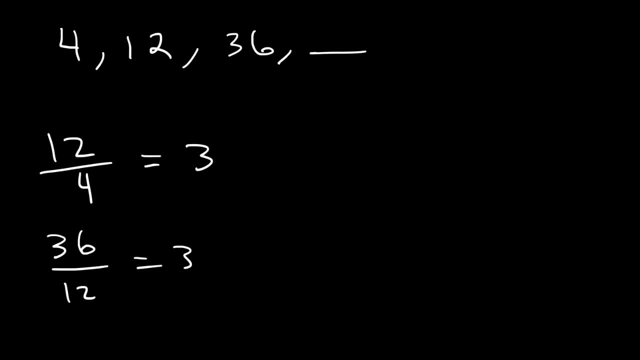 by 12 is 3.. So we have a common ratio. If we multiply 4 by 3, it will give us 12.. And if we multiply 12 by 3, that will give us 36.. So to find the next number in the sequence: 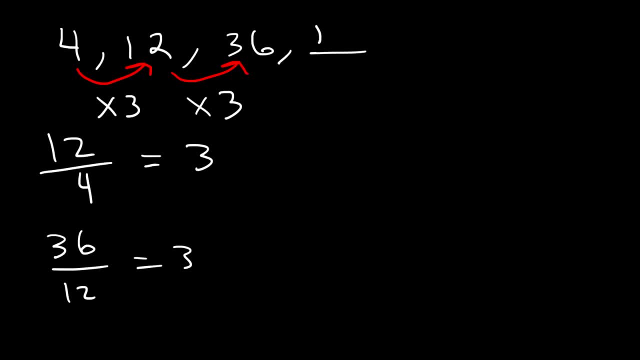 we've got to multiply 36 by 3, and that's going to give us 108.. And if we want to find the next two numbers, we'll need to continue to multiply by 3.. 108 times 3 is 324, and 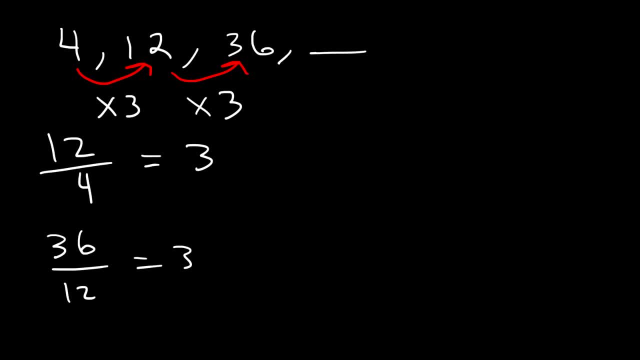 So to find the next number we've got to multiply thirty-six by three, and that's going to give us a hundred and eight. And if we want to find the next two numbers we'll need to continue to multiply. So that's going to give us a hundred and eight. 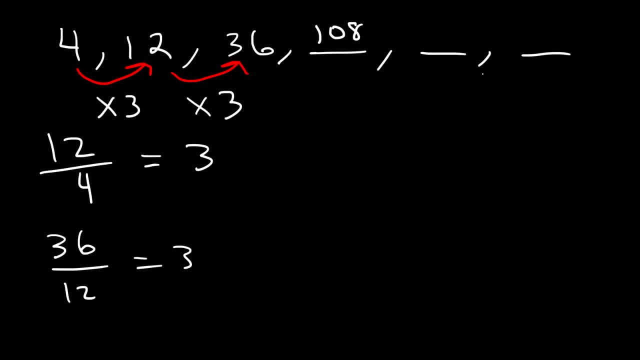 And to continue to multiply by three. one-oh-eight times three is three-twenty-four, and three-twenty-four times three is nine-seventy-two, And so that's it for this example. Go ahead and find the missing numbers in the sequence. 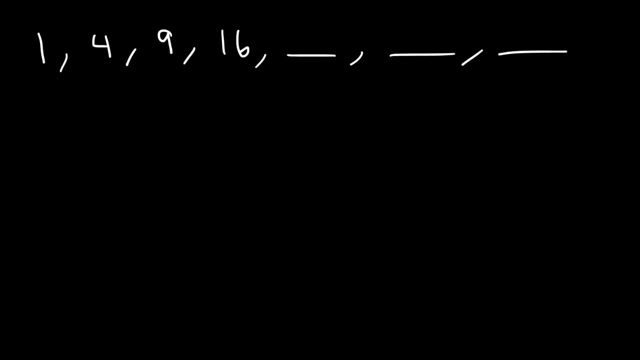 So feel free to pause the video to find the answer. If we look at the first example, One squared is the same as one. two squared is four. three squared is nine. four squared, or four times four, that's sixteen. So the next number has to be five squared, which is twenty-five. 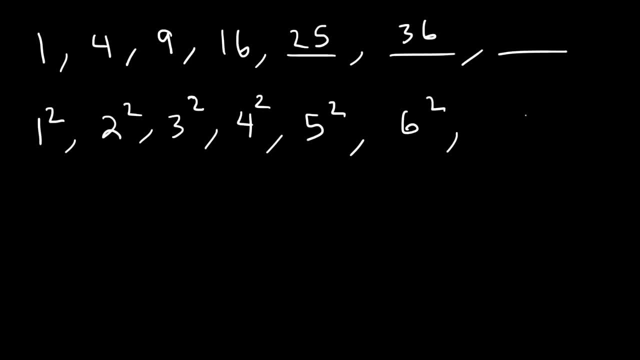 And then it's six squared, which is thirty-six, and seven squared, which is forty-nine. So look out for exponents, because sometimes you might have that as a pattern. Try this: one, Eight, twenty-seven, sixty-four, And then go ahead and find the missing numbers. 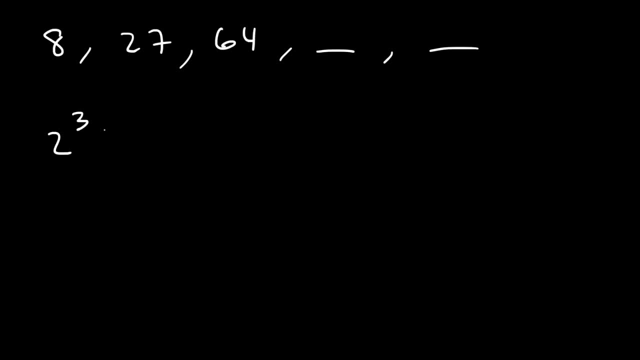 Now, eight is the same as two to the third. Two times two times two is eight. Twenty-seven is three to the third, Four to the third, or four times four times four, that's sixty-four. Therefore, the next number in the sequence has to be five to the third, which is one-twenty-five. 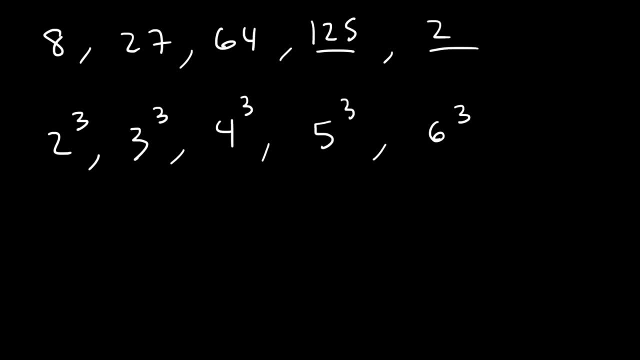 So that's sixty-four, And then we have six cubed, which is two-sixteen, And the next one will be seven to the third, and then so forth. Find the pattern. Consider the sequence: four, six, nine, thirteen and eighteen. 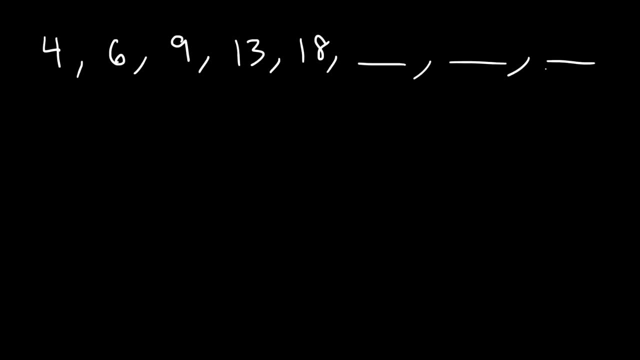 So go ahead and find the next numbers. Well, we're not dealing with exponents here, Because six, thirteen and eighteen, Those are not perfect squares or perfect cubes. So let's see if there's a common difference or a common ratio. 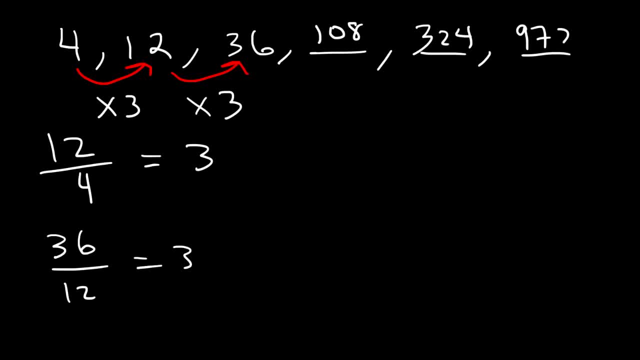 324 times 3 is 972.. And so that's it for this example. Go ahead and find the missing numbers in this sequence. So feel free to pause the video to find the answer. If we look at the first example, 1 squared is the same as 1.. 2 squared is 4.. 3 squared: 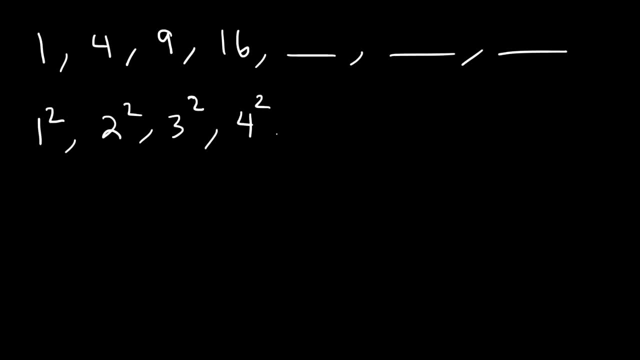 is 9.. 4 squared, or 4 times 4,, that's 16.. So the next number has to be 5 squared, which is 25.. And then it's 6 squared, which is 36.. And 7 squared, which is 49.. So the next number 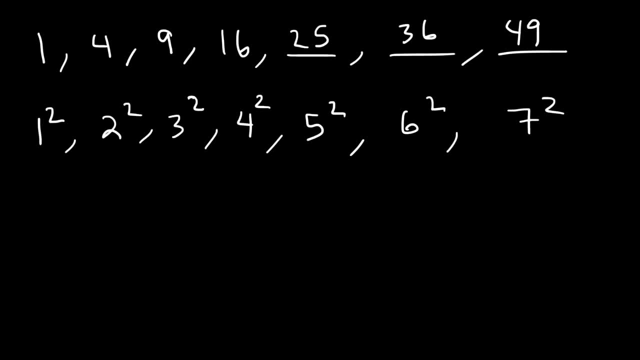 is 9.. So look out for exponents, because sometimes you might have that as a pattern. Try this one: 8,, 27,, 64. And then go ahead and find the missing numbers. Now, 8 is the same as 2 to the 3rd, 2 times 2 times 2 is 8.. 27 is 3 to the 3rd, 4 to the 3rd or 4 times. 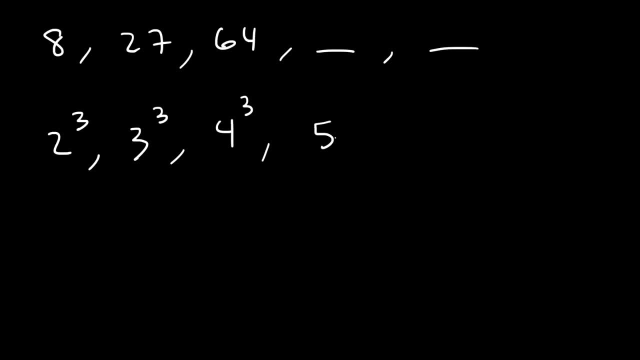 4, that's 64. Therefore, the next number in the sequence has to be 5 to the 3rd, which is 125.. And then we have 6 cubed, which is 216.. And the next one will be 7 to the 3rd. 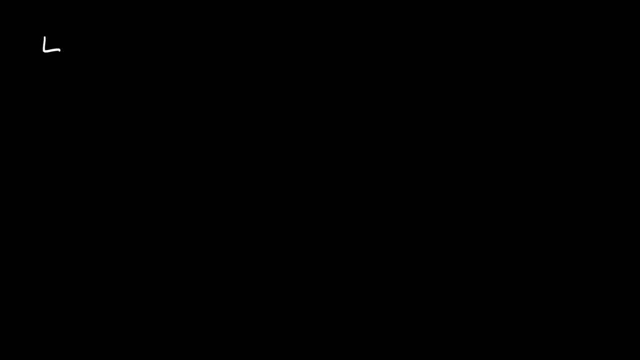 and then so forth. Find the pattern. Consider the sequence: 4,, 6,, 9,, 13, and 18.. So go ahead and find the next numbers. Well, we're not dealing with exponents here, because 6,, 13, and 18, those. 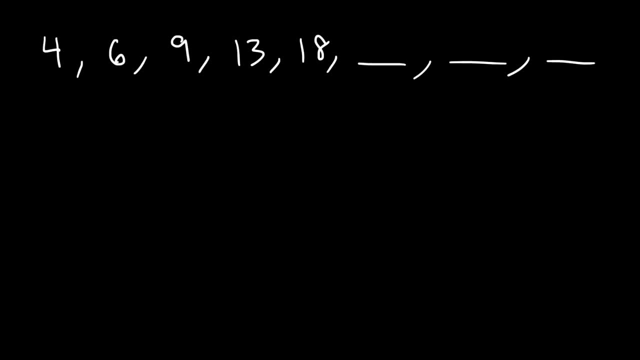 are not perfect squares or perfect cubes. So let's see if there's a common difference or a common ratio. Now, if we subtract 6 by 4, that will give us 2.. And if we divide 6 by 4, that's 1.5.. 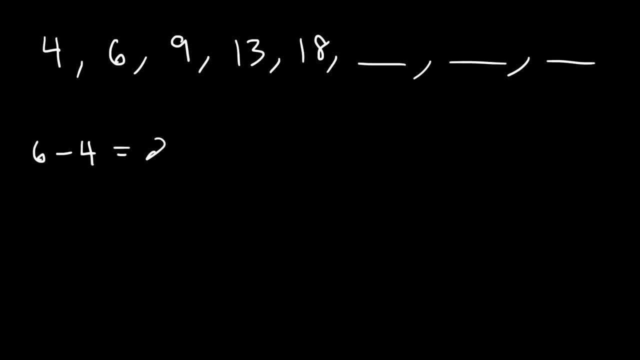 Now, if we subtract six by four, that will give us two, And if we divide six by four, that's one-point-five. If we subtract nine by six, that will give us three, And if we divide nine by six, that's also one-point-five. 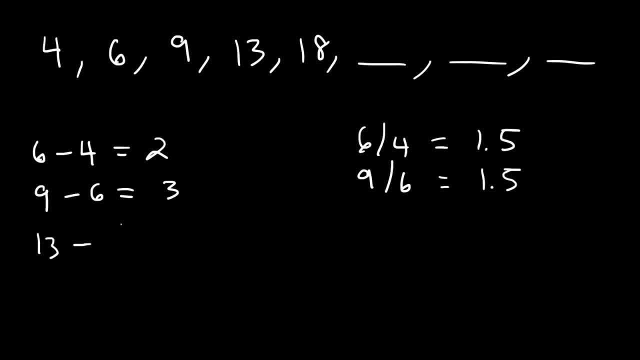 5. if we take 13 and subtracted by 9, that's 4, and if we take 13 and divided by 9, it's no longer 1.5, it's actually 1.444. repeating now, if we take 18 and 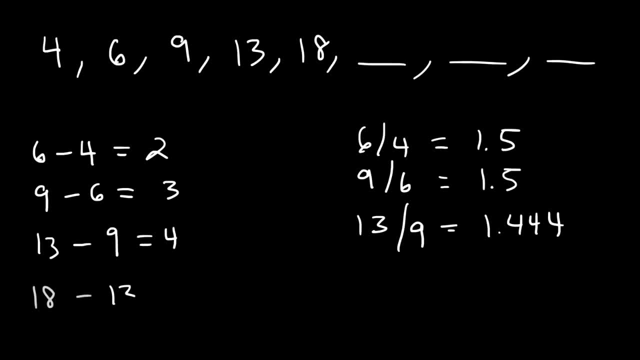 subtracted by 13, that gives us 5, and if we take 18 and divided by 13, that's one point. three, eight, four, six. now notice that with division there is no pattern that we can use here, but with subtraction there is a pattern, even. 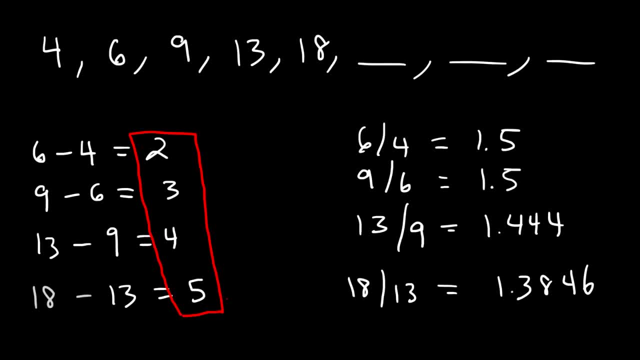 though we don't have a common difference, the difference is increasing by one. so to go from 4 to 6, we need to add 2, and to go from 6 to 9, we need to add 3. to go from 9 to 13, we got to add 4, and to go to 13 to 15, we need to add 5. so 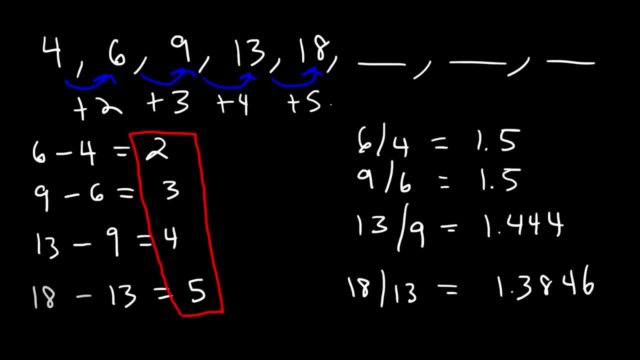 therefore, the next number has to be 18 plus 6, which is 24, and then after that we need to add 7. 24 plus 7 is 31, and then we need to add 8. 31 plus 8 is 39. so, based on the pattern, 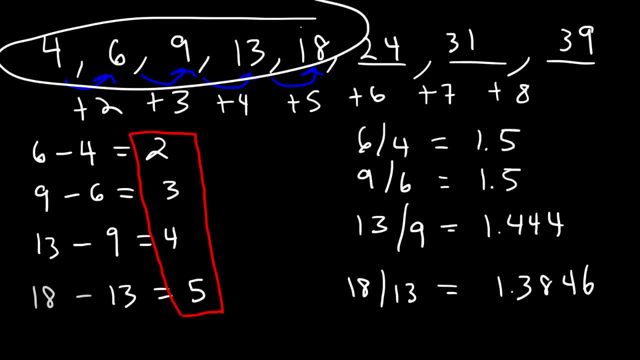 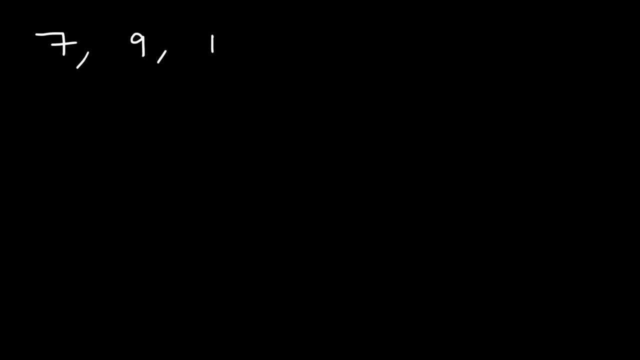 that we see here. that's how we could find the next set of numbers. here's another example: 7, 9, 13, 19, 27. using those five numbers, find the next three numbers. so what is the difference between 7 and 9? if we take 9 and subtracted by 7, we're. 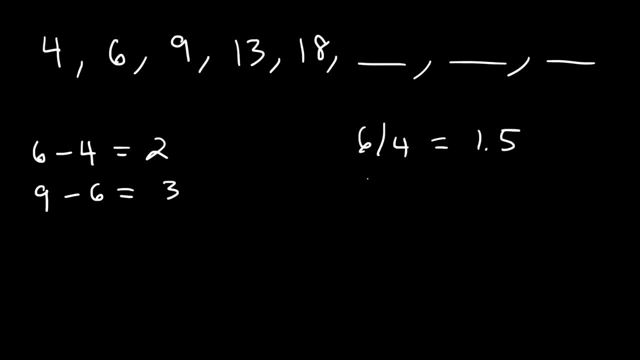 If we divide 9 by 6, that will give us 3.. And if we divide 9 by 6, that's also 1.5.. If we take 13 and subtract it by 9, that's 4.. And if we take 13 and divide it by 9, it's. 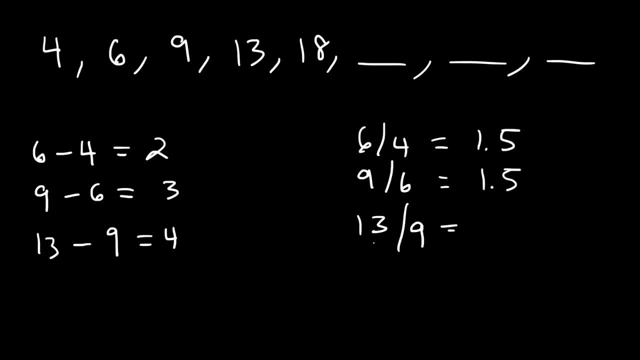 no longer 1.5.. It's actually 1.444.. Repeat it Now: if we take 18 and subtract it by 13,, that gives us 5.. And if we take 18 and divide it by 13,, that's 1.3846.. Now notice that with division there is no pattern that we 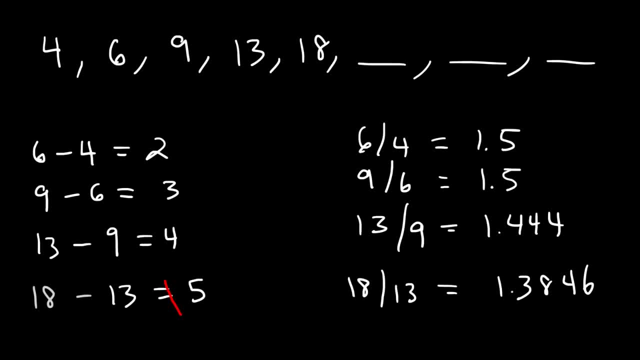 can use here. But with subtraction there is a pattern. Even though we don't have a common difference, The difference is increasing by 1. So to go from 4 to 6, we need to add 2. And to go, 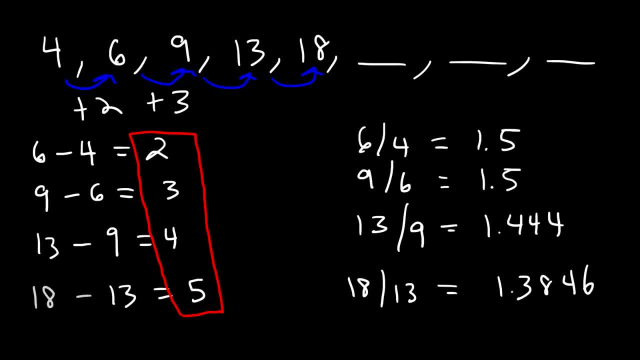 from 6 to 9,, we need to add 3.. To go from 9 to 13,, we got to add 4.. And to go to 13 to 15,, we need to add 5.. So, therefore, the next number has to be 18 plus 6,, which is: 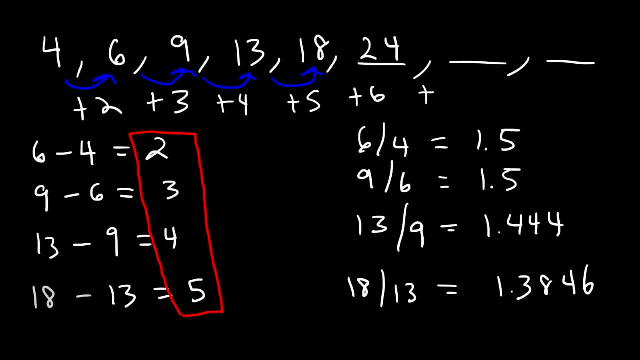 24.. And then after that we need to add 7.. 24 plus 7 is 31.. And then we need to add 8.. 31 plus 8 is 39. So, based on the pattern that we see here, that's how we could define. 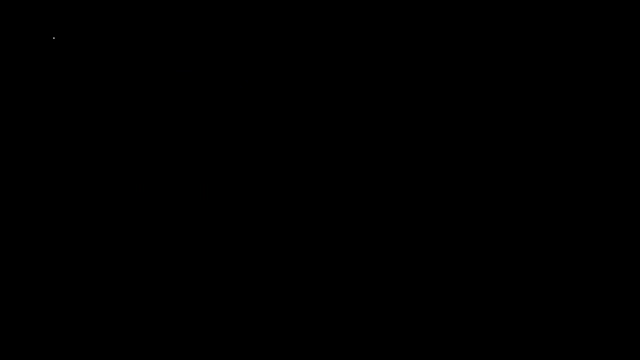 the next set of numbers. Here's another example: 7, 9,, 13,, 19, 27.. Using those five numbers- five numbers- we find the next three numbers. So what is the difference between 7 and 9?? 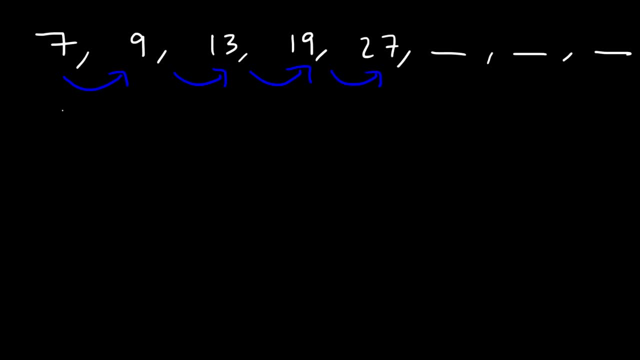 If we take 9 and subtract it by 7, we're going to get a difference of 2.. If we take 13 and subtract it by 9, we're going to get a difference of 4.. 19 minus 13 is going to be a difference. 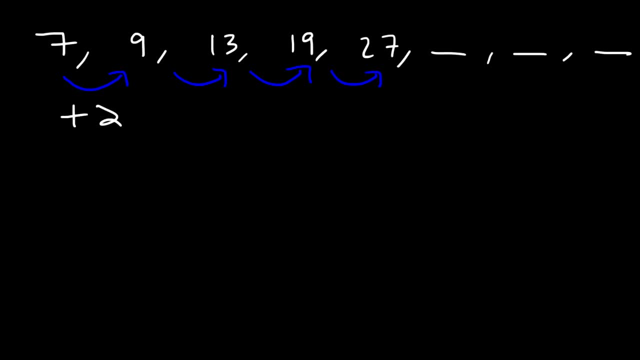 going to get a difference of 2. if we take 13 and subtracted by 9, we're going to get a difference of 4: 19 minus 13 is going to be a difference of 6, and 27 minus 19 is a difference of 8. so therefore, in order to find the next, 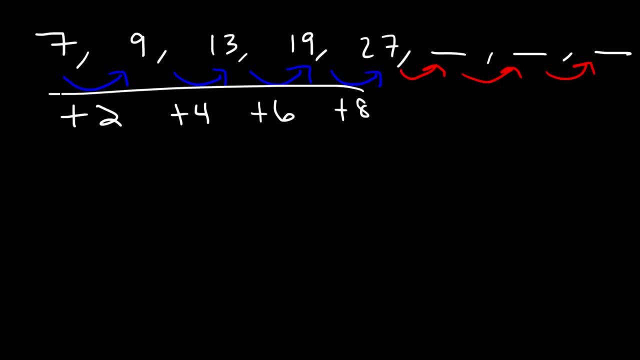 number. we can follow the sequence here. the sequence of addition increases by 2, so next time we get to add 10, 27 plus 10 is 37, and then we need to add 12. 37 plus 12 is 49, and then we'll add 14, 49 plus. 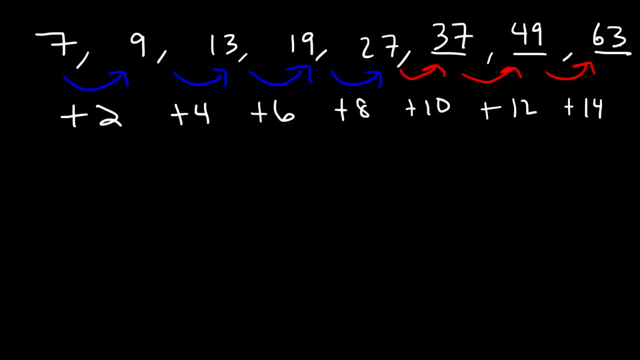 14 is 63, and so that's it. that's how you can find the next three numbers. sometimes you need to see the pattern in a fraction. So let's say, if we have these four fractions- 3 over 4,, 5 over 7,, 7 over 10, and 9 over- 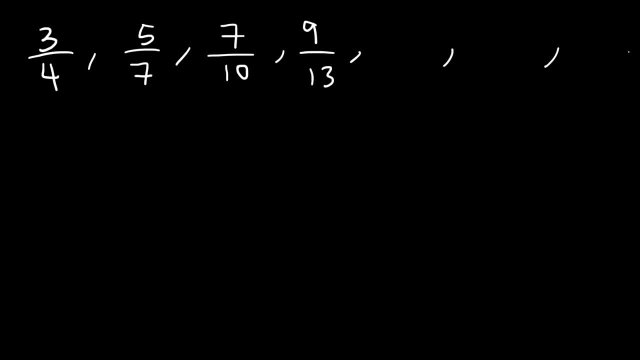 13. So, based on this, find the next three fractions. So how do we do this? How would you begin? So take a minute and see if you can figure this out Now. when dealing with fractions, personally I find it helpful to separate the numerator. 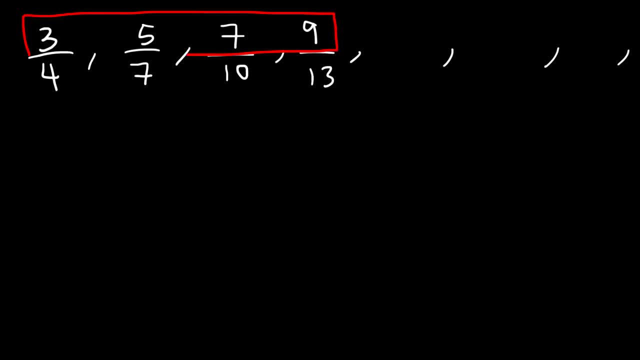 and the denominator. If we focus on the top numbers, we could see a pattern between 3,, 5,, 7, and 9.. The common difference between those numbers is 2.. 3 plus 2 is 5,. 5 plus 2 is 7,. 7 plus 2 is 9.. 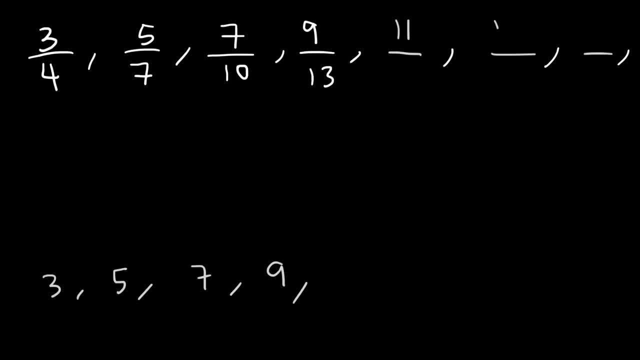 So, therefore, the next three top numbers have to be 11,, 13, and 15.. Now let's focus on the denominator 4,, 7,, 10, 13.. Notice that each of those numbers differ by 3.. 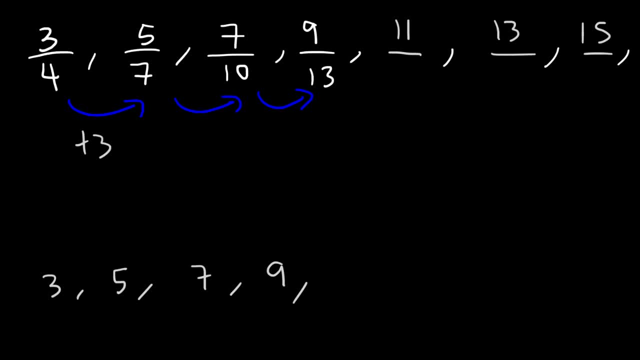 4 plus 3 is 7,, 7 plus 3 is 10,, 10 plus 3 is 13,. so 13 plus 3 is 16, and then we have 19,, and then 19 plus 3 is 22.. 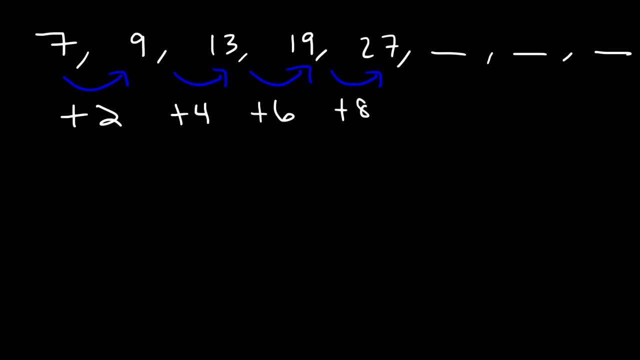 of 6. And 27 minus 19 is a difference of 8.. So therefore, in order to find the next number, we can follow the sequence here. The sequence of addition increases by 2.. So next time we're going to add 10.. 27 plus 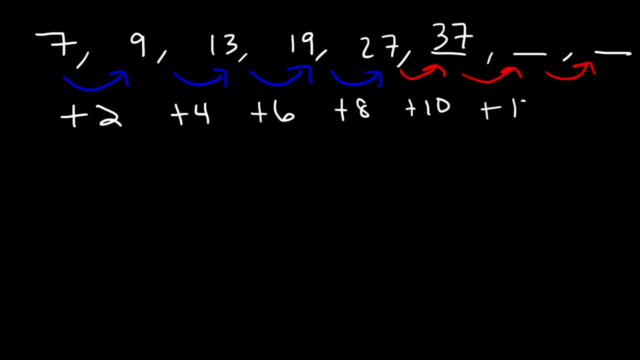 10 is 37. And then we need to add 12.. 37 plus 12 is 49. And then we'll add 14.. 49 plus 14 is 63. And so that's it. That's how you could find the next three numbers. Sometimes you need. 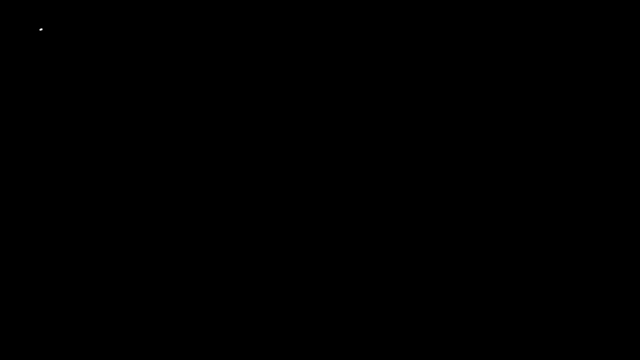 to see the pattern. So let's say we have these four fractions: 3 over 4,, 5 over 7,, 7 over 10, and 9 over 13.. So, based on this, find the next three fractions: 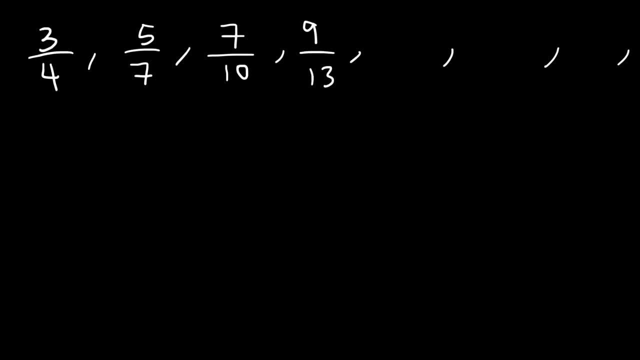 So how do we do this? How would you begin? So take a minute and see if you can figure this out Now. when dealing with fractions, personally, I find it helpful To separate the numerator and the denominator. If we focus on the top numbers, we could see a pattern between 3, 5,, 7, and 9.. 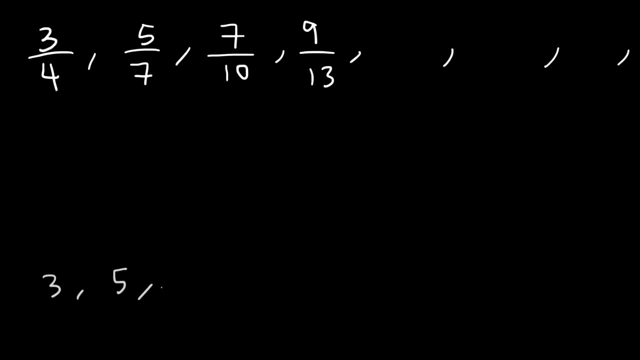 The common difference between those numbers is 2.. 3 plus 2 is 5.. 5 plus 2 is 7.. 7 plus 2 is 9.. So therefore the next three top numbers have to be 11,, 13, and 15.. 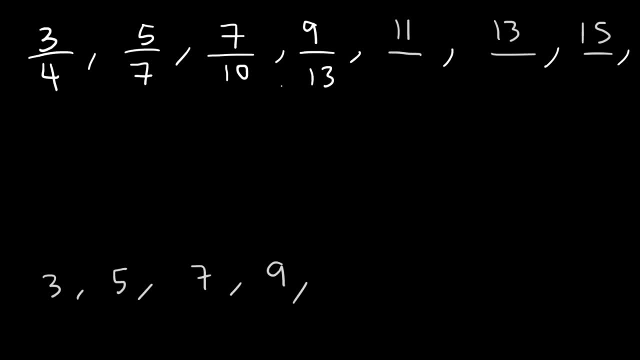 Now let's focus on the denominator. Let's focus on the denominator 4,, 7,, 10, and 13.. Notice that each of those numbers differ by 3.. 4 plus 3 is 7,, 7 plus 3 is 10,, 10 plus 3 is 13,. so 13 plus 3 is 16, and then we have 19,. 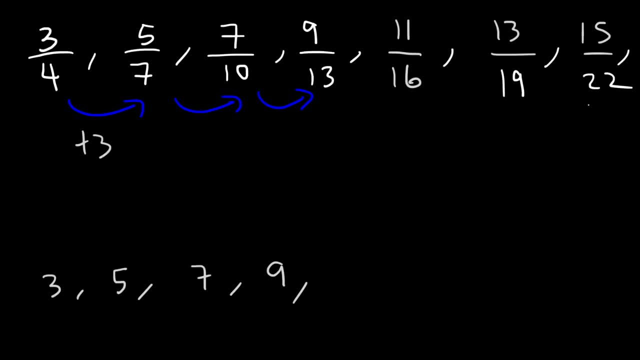 and then 19 plus 3 is 22.. And so you want to separate the fractions into the top and the bottom portion. Just see it separately And it can help you to figure out the missing terms. Here's another example: 11 over 4,, 8 divided by 9,, 5 over 16..